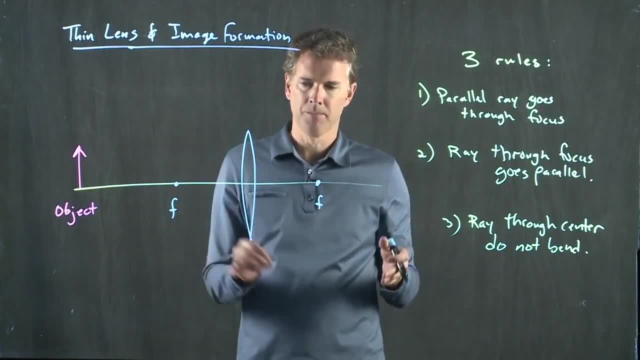 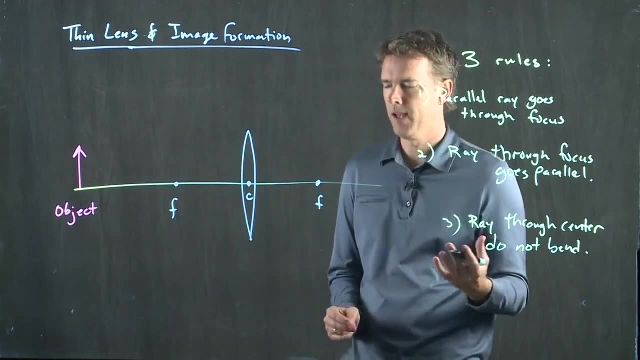 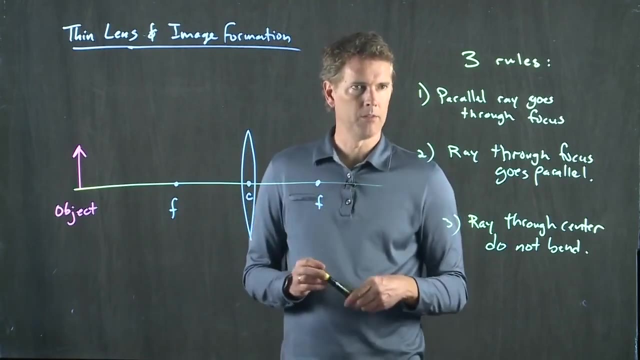 for a curved mirror, It was the center of that radius of curvature, But here, for a thin lens, the center is in fact, right in the center of the lens. Okay, All right, so let's see how to do this. We've got our object. We need to draw some of these rays. The first one is parallel ray goes. 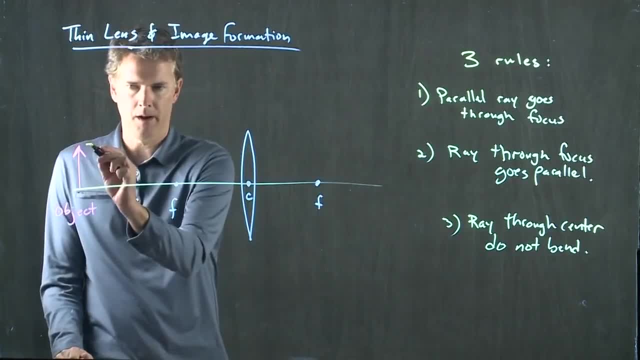 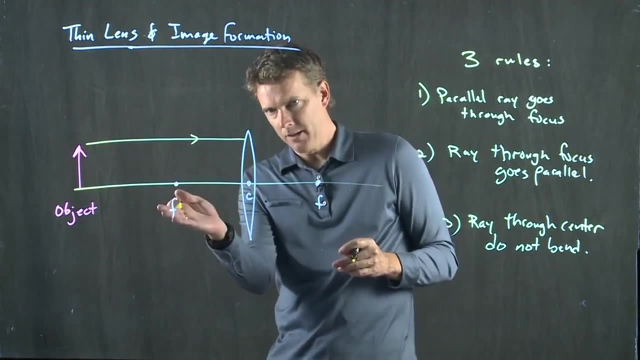 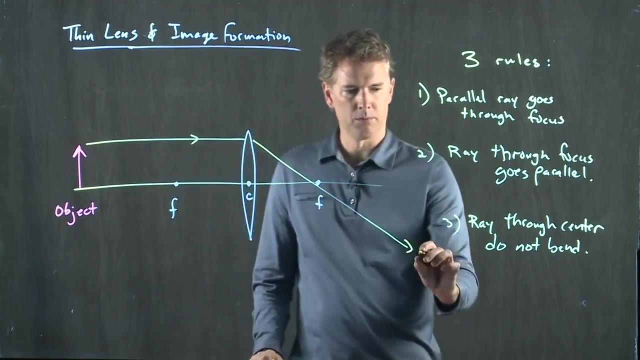 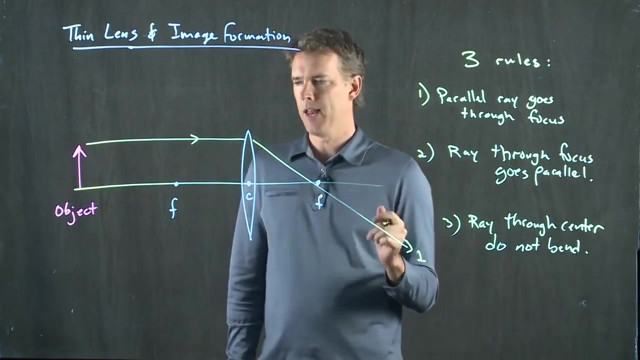 through the focus. Okay, Parallel ray comes in. It's going to go through the focus. It's not going to bounce off this glass and go back to this focus. It's going to bend and go through this focus. Okay, so this is ray number one. Ray number two is going through the focus. It then goes parallel. 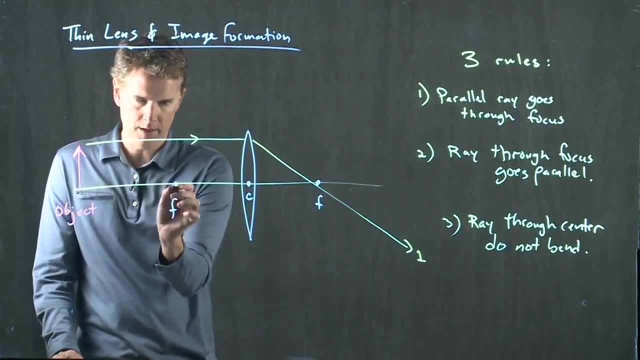 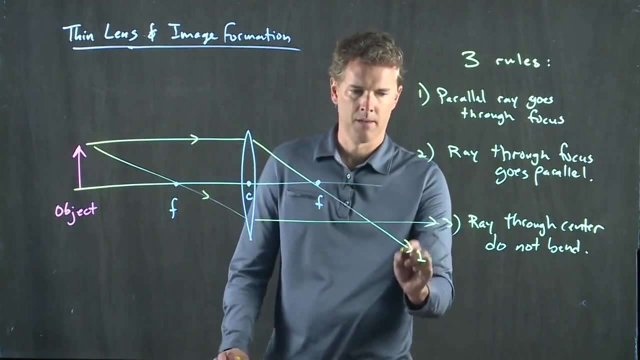 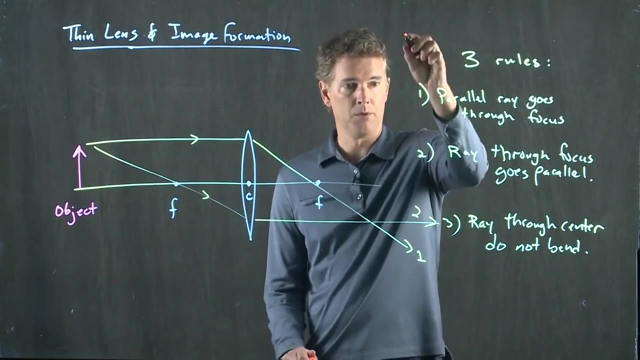 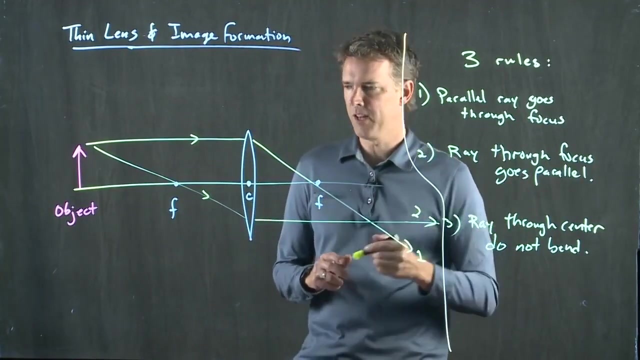 All right, Going through this focus, It then goes Parallel. This is ray number two, And then, finally, there we'll draw a little separator right here there. Finally, we have rule number three, which is raise through the center, do not. 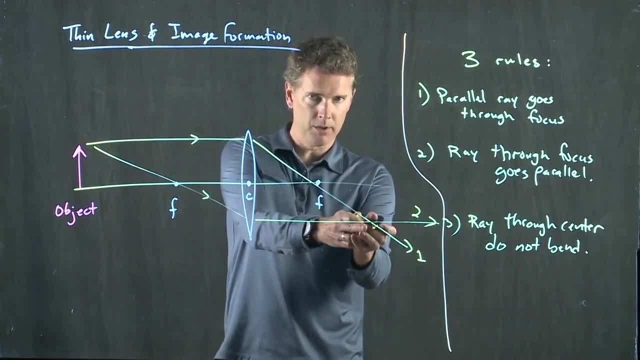 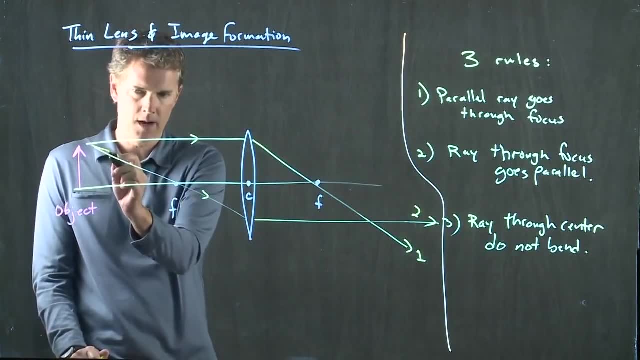 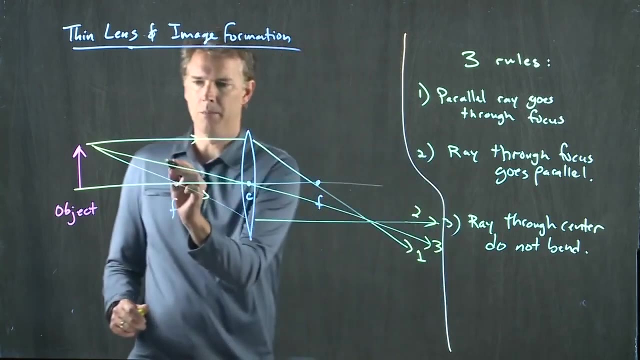 bend. Now we already have an intersection point, so you really only have to do two of these three. But just for kicks, let's draw the third one and make sure it works out. Raise through the center, do not bend. That's ray number three. Okay, And these are reasonably 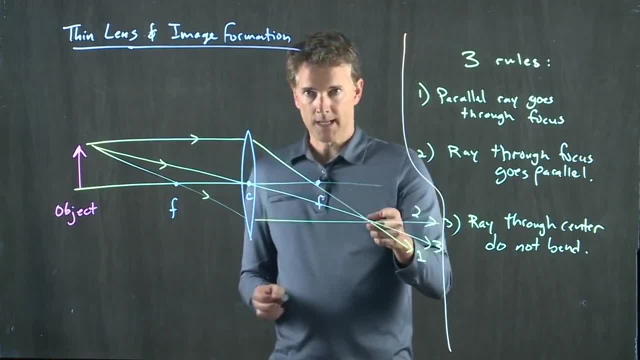 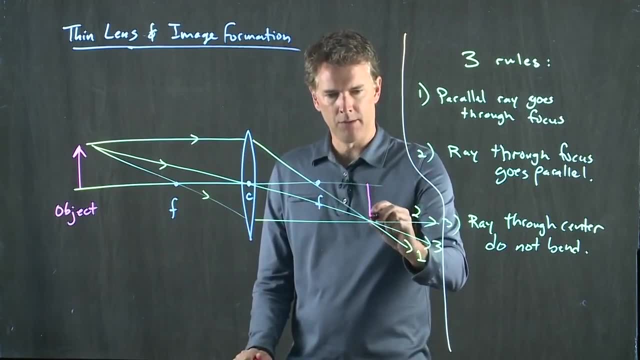 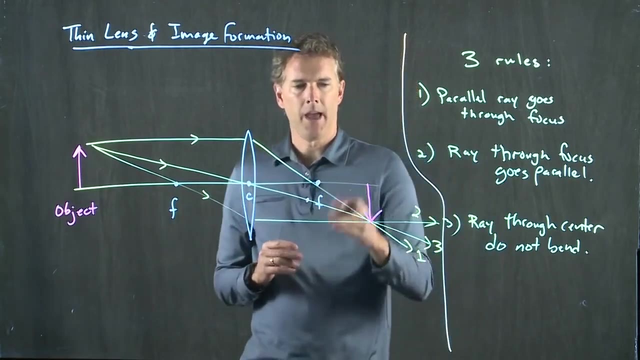 straight. That's where the object generates an image. We know that the base of the object is still going to be on the optical axis, and so it is inverted. In this case, it looks like it is demagnified, and that is where the image is located. Okay, So those are the 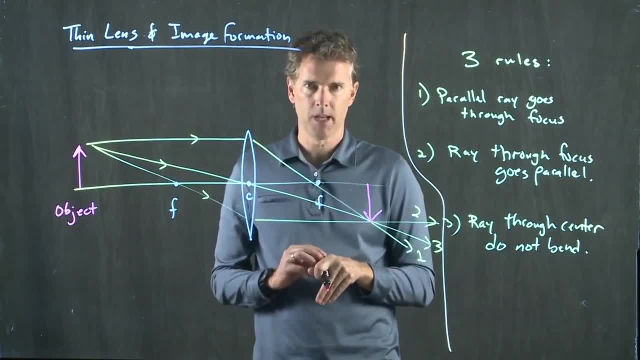 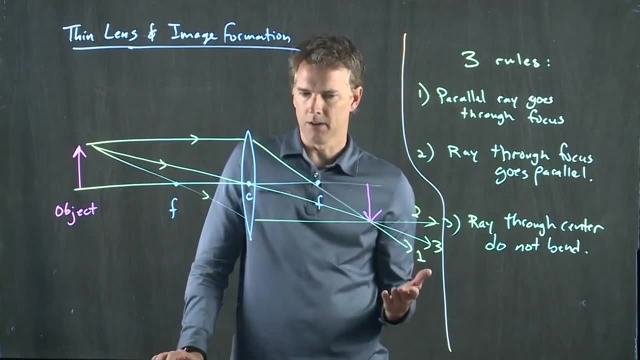 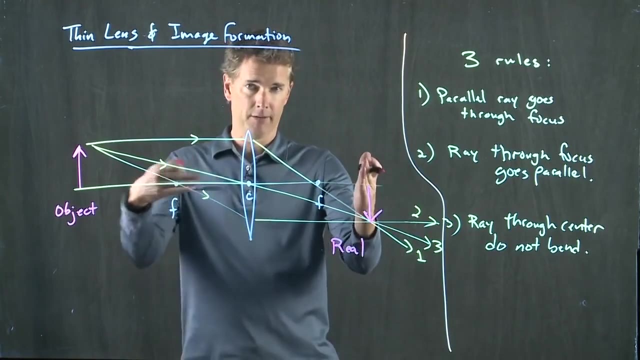 three rules for figuring out where that image is located. And it takes a lot of practice and as you move this up, If you move this object in and out, it gets a little bit harder and harder to do. This is a real image. In other words, if I put a piece of paper there, I can form an image.